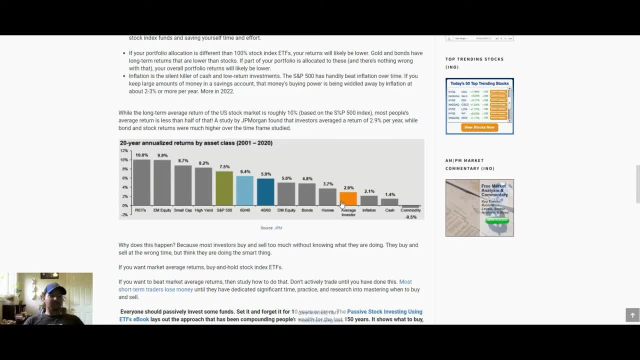 knew what they were doing but not knowing what they were doing. So if you're just an average investor looking to get long-term returns, it's really best to just ride out the ups and downs in the stock market, even though we are going to have those big years where it goes up a lot and we have those years where it goes down a lot. But over the long term the returns are great if you're invested in the stock market. So this just shows trying to 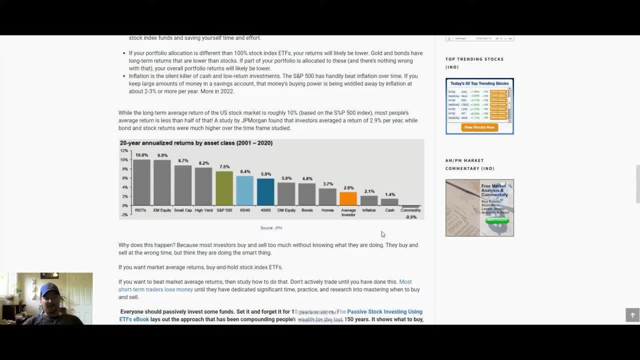 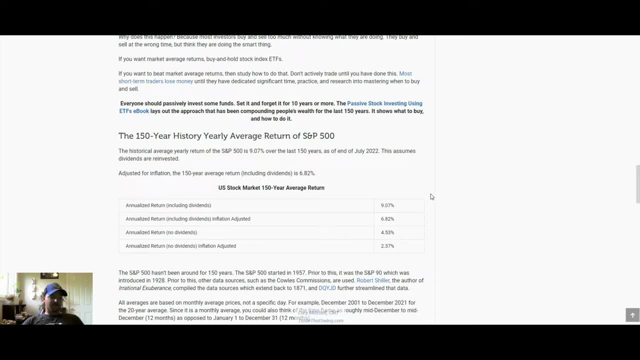 trade in and out, in and out, in and out. it's probably not the best if you don't know what you're doing. So over the last 150 years, the return including dividends, and we want to note that big difference there If we don't include dividends. your returns about 4.5%. If you include dividends and you take those dividends and you reinvest them back into your portfolio- so you're taking those dividends and just buying more S&P 500 ETF- then the return is nine point seven percent. so that's a hundred hundred and fifty years worth of 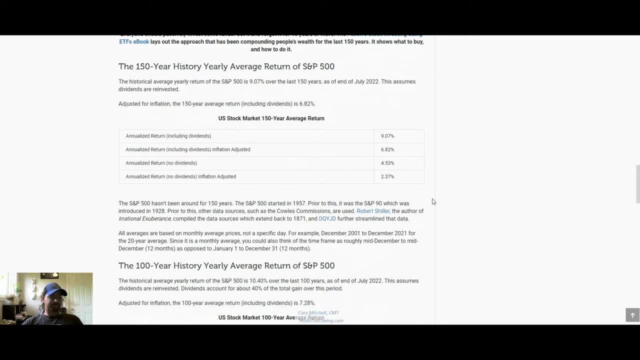 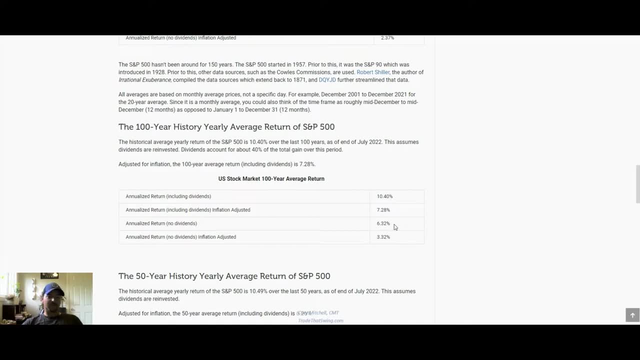 returns. that's your average over the last hundred years. it's a little bit better. ten point four percent. again, you notice the big difference there. if you don't, if you just take your dividends out and spend them, you're gonna have quite a bit less per year. then if you reinvested those dividends and that's. 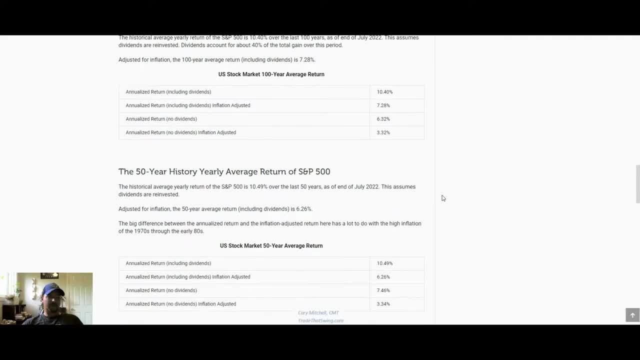 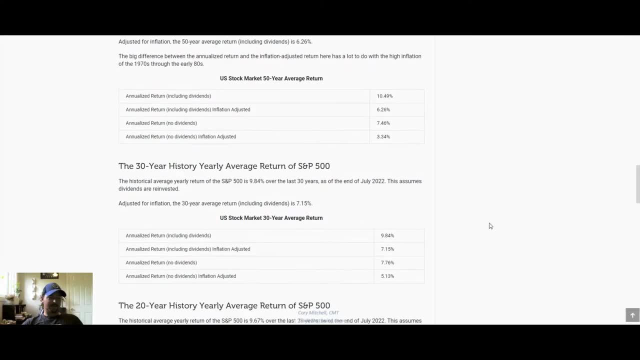 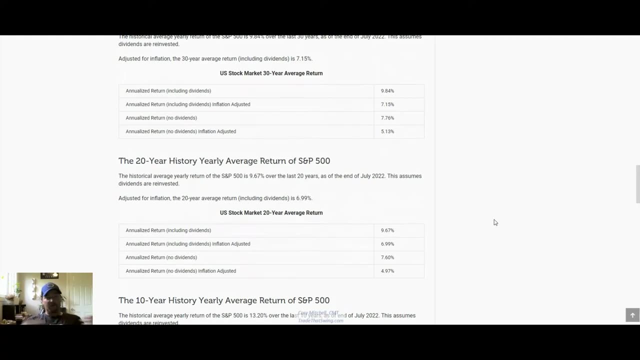 just the compounding effect over time. last fifty years about the same ten point, five percent. thirty years pretty close to that ten percent. again last 20 years still having around that ten percent mark. so even though we do we know we have up and down years, it still averages out to ten percent a year. so 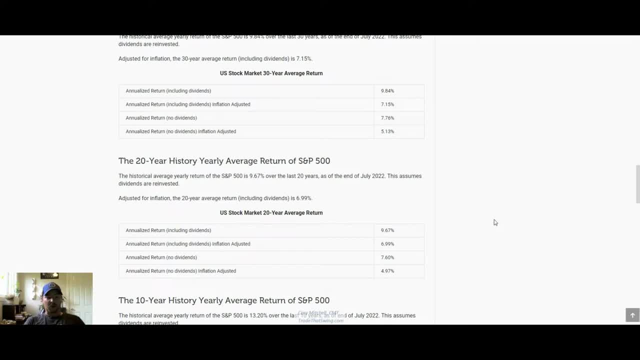 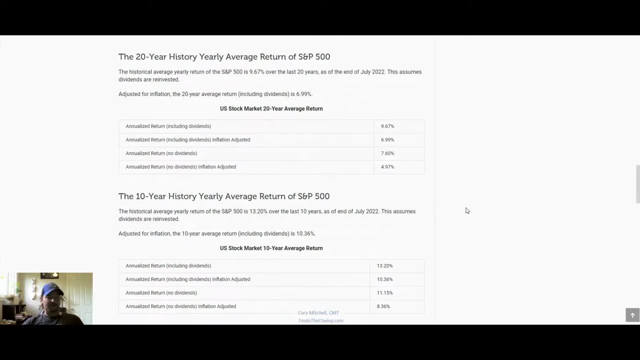 you're gonna have a couple down years. you're gonna have a couple down years. so you're gonna have a couple down years. you're gonna have some up years, but overall this is what we end up with. shorter term, we can have bigger fluctuations because each year becomes. 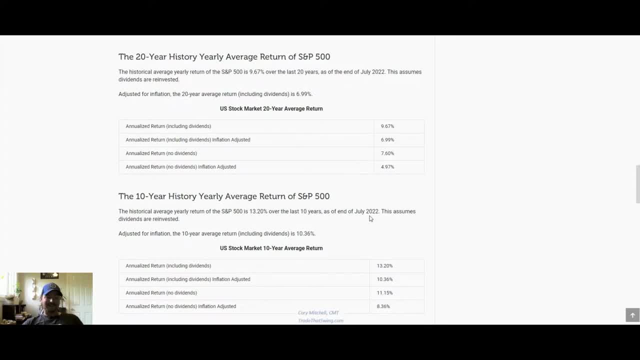 more important over the last ten years. this was as of the end of July and all these figures are calculated based on monthly average prices, so it's not going right up to the end of July is taking the average price of all July 2022. so thirteen point two percent, that was a pretty big year. 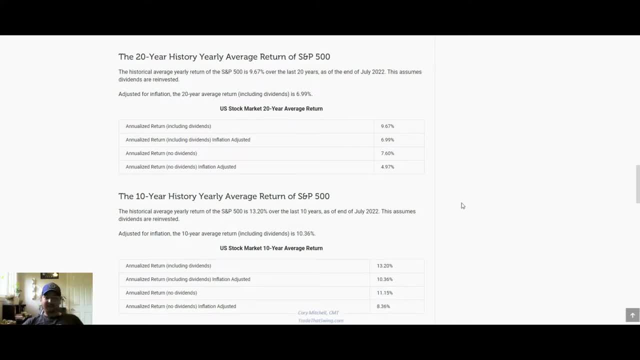 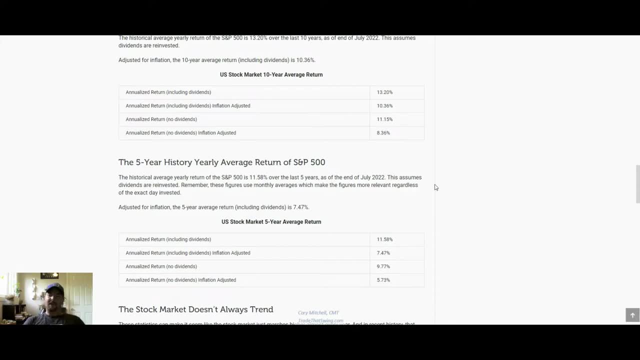 or pretty big decade for stocks. that's a. it's a nice high return overall and short-term we're not going to worry about those as much, assuming you have somewhat of a longer time horizon- ten years, twenty years- we can hopefully assume that that ten percent a year, which has been pretty dominant over the 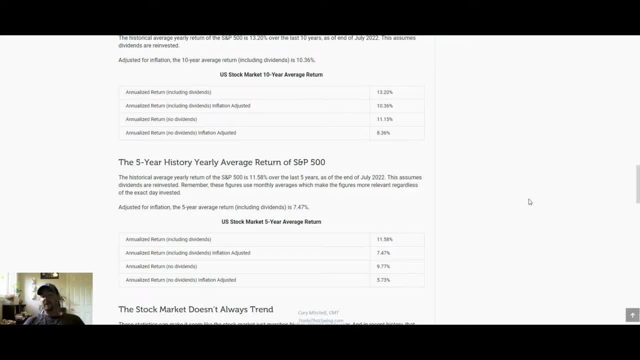 last hundred and fifty years will continue to hold, although there's no way to know that. we're looking at historical data. the average has been 10%. whether that continues to hold or not is not clear yet into the future. we don't know. but it's a pretty good benchmark to go off of. so 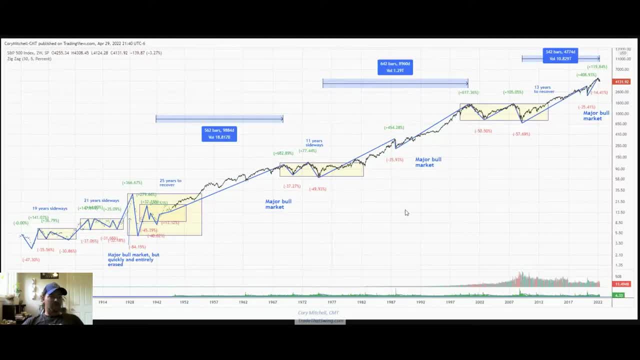 the stock market doesn't always trend, though. there are going to be periods where we have sideways movement. most of us were alive during the either the dot-com crash or the financial crisis of 2008-2009, and we can see there was a period here where, if you had invested back in 2000, it took a while for you to. 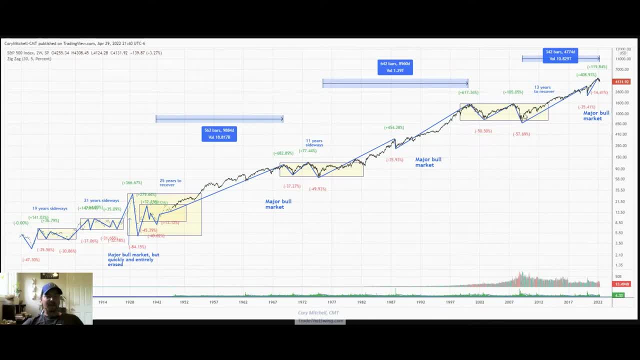 recover those losses. so it dropped, came back, dropped again, came back. so this was about 13 years of what we could consider overall sideways movement. now I generally encourage people: if you're an investor, just invest a little bit each month. that way you have been buying all the way down here and you you have had a 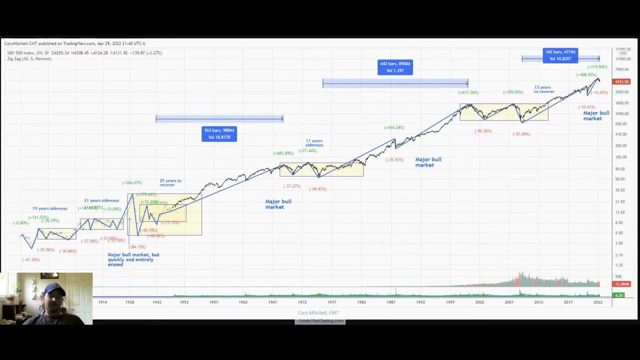 much quicker recovery and buying a little bit on the drop and you would have been buying as the price recovered. so your recovery point would have actually been the half way waypoint of this 13 year period. so quite a bit of this time you would have been seeing some nice. 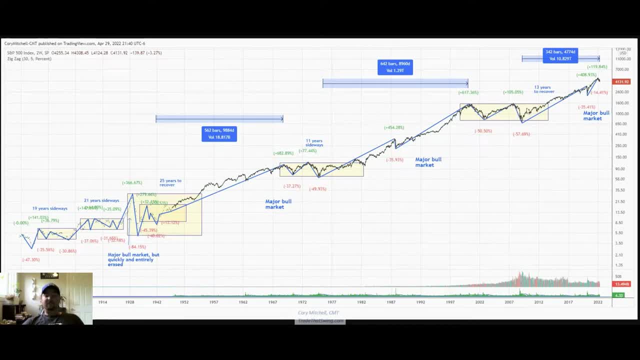 gains, plus you would have been getting dividends and then eventually we had a very nice run after that. so the same thing has happened multiple times before. if we go back to the 19, late 1960s, 1970s, same thing. basically one big drop. we recovered nice big drop again, and then we recovered big drop. 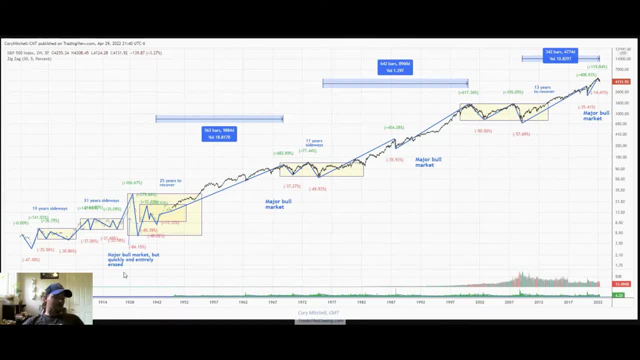 big drop, recover. same thing, even though it was much bigger initial drop. the same thing happened back in the 30s. we had this massive rise and the big sell-off in the late 1920s rallied, didn't quite get back to the peak like we did in these other ones, but then we also didn't sell off right. 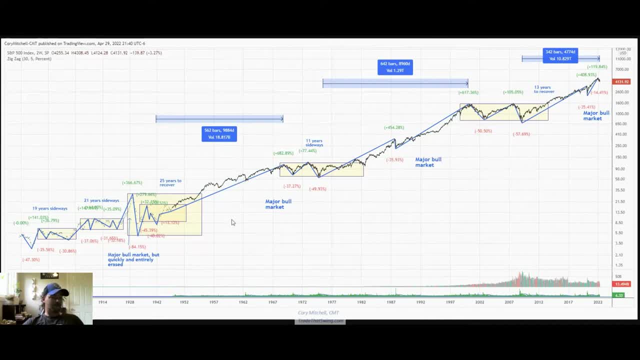 to the bottom either. so basically two big drops and then the recovery. if we even go back into the early 1900s: big drop, recovery, big drop, again recovery. same thing happened in even earlier in the 1800s- big drop, recovery, big drop. so we we have these periods where we tend 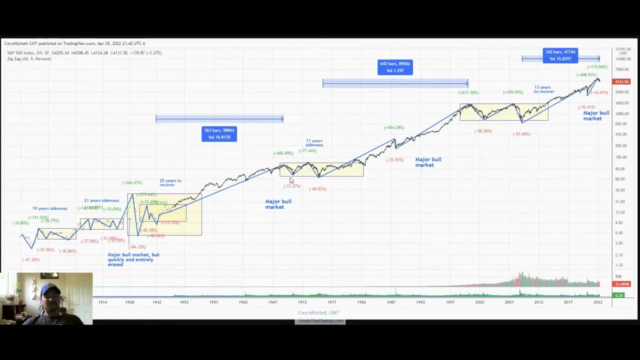 to have two pretty sizable drops which during those times stocks move sideways for about 10 years and took a little bit longer, almost 25 years, for the stock market to recover after the Great Depression and this massive decline. but again, if you'd been buying throughout this time, the 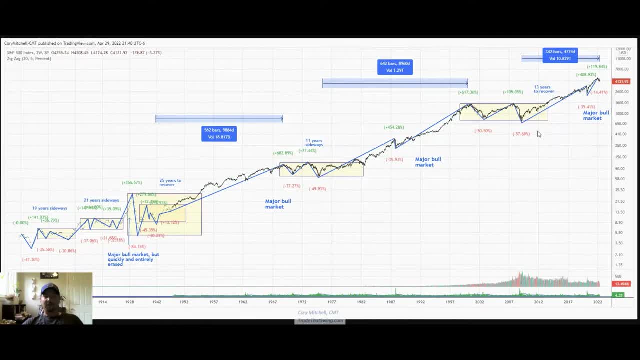 recovery would have been much quicker. you would have started to recover once this was recovering about halfway up this range, as opposed to waiting all the way till it made new highs. so as investors, even though there are these big declines, we can still make good returns even during these periods and will do very well during these big trending. periods, so that 10% average encompasses all of this and encompasses the big declines and it encompasses the big rallies. and that's what we want to keep in mind with our big picture. thinking of what returns could be if you're just invested in an S&P type fund to give. you some perspective. what are the biggest up and down years in the S&P 500? well, if we go back to 1928, there was the biggest up here. it was forty six point five, nine four, forty six point five, nine percent, and that was just after the Great Depression, so, or as we were recovering from it. 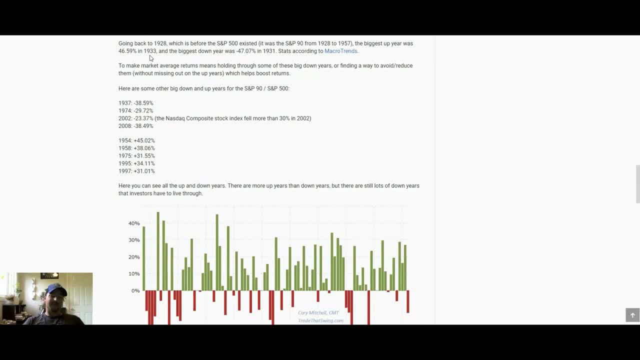 so sometimes from these big declines you get the biggest rallies. so it can be your timing has to be perfect if you're trying to step out and then step back in, because if, if you miss one of those big moves you could be in for you know, your statistics could be much different than what. 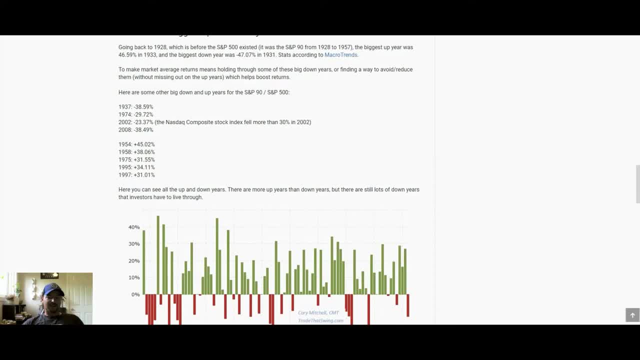 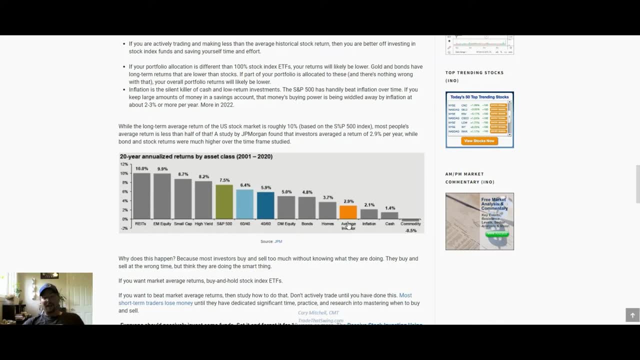 the long-term averages are and, as we discussed, you don't want to be one of these people who's trying to avoid all the bad times and only get in for the good times, and what usually happens is that you miss some of the good times as well, and that's why you end up with the low return. so biggest up here or biggest down here was forty seven percent in one year in 1931, some of the other notable years. just to know, just if you're gonna be holding S&P type hundred fund, these are some of the returns you could see in a given year. you could see a forty percent drop, a thirty percent. 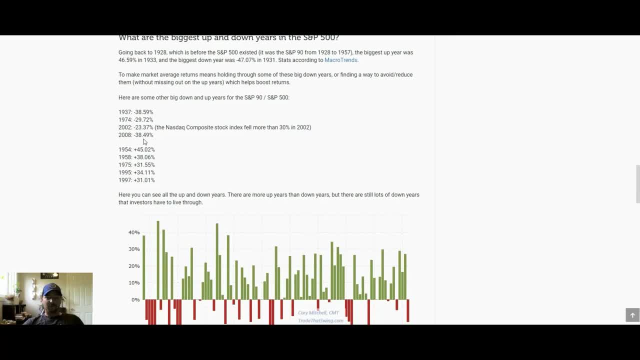 drop. a twenty three percent drop. two thousand eight hundred percent drop. twenty three percent. almost thirty nine percent drop, pretty significant. if you're watching that it is a gut-wrenching. but we also have to remember that we have up here is a forty five percent thirty eight percent thirty. 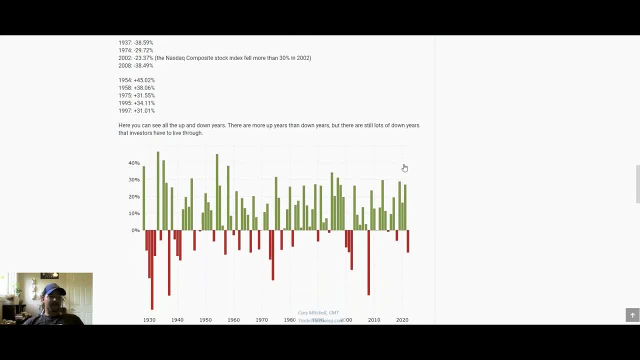 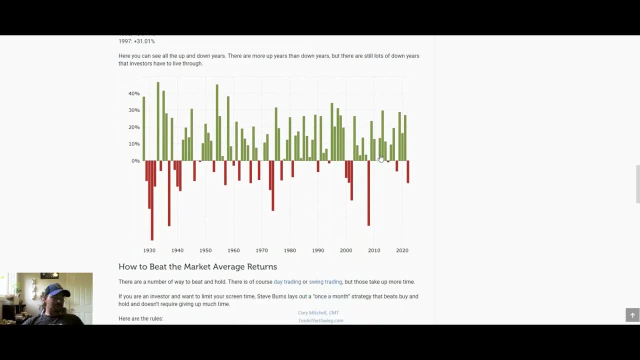 one percent. ninety seven was thirty one percent rally and you can see the dispersion here where we can see slightly more appears than down years, probably about sixty percent up years, just eyeballing it, and thirty to forty percent down years. we have some that are pretty much flat, you could say where it's just a minor loss or a minor game. we have some pretty big downside. 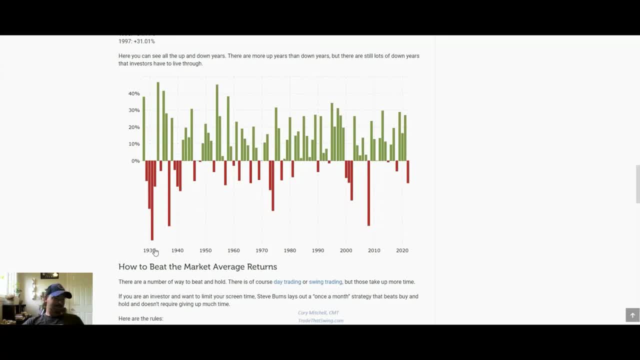 years, but when you look at this, this is a almost 90 year time span. we're looking at here from 1930 to 2020 and just beyond. there's a few big down years, but not a whole lot, and there's a lot of kind of average up years and then we have a few really big up years, and this is what the typical 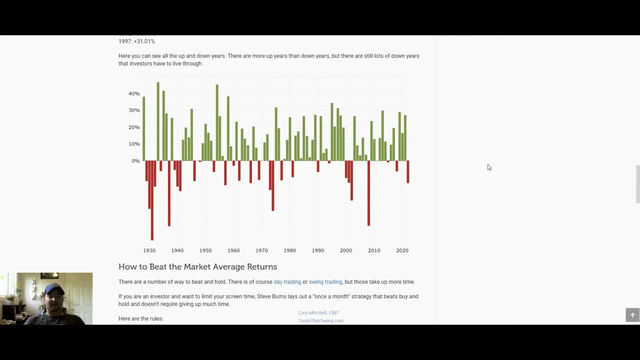 dispersion looks like. so when we say that the stock market is up an average of ten percent per year, that doesn't mean it's just gonna go up ten percent a year and your thousand dollar portfolio is going to be worth eleven hundred next year and then ten percent on that the next. 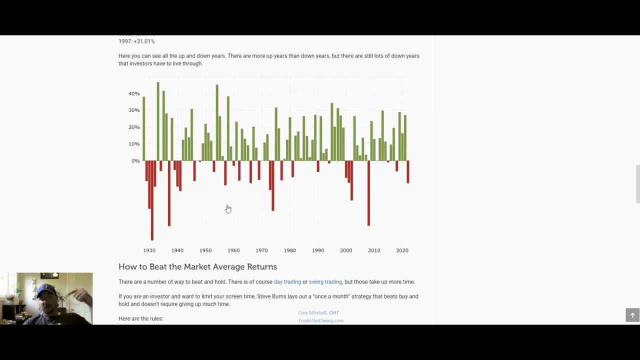 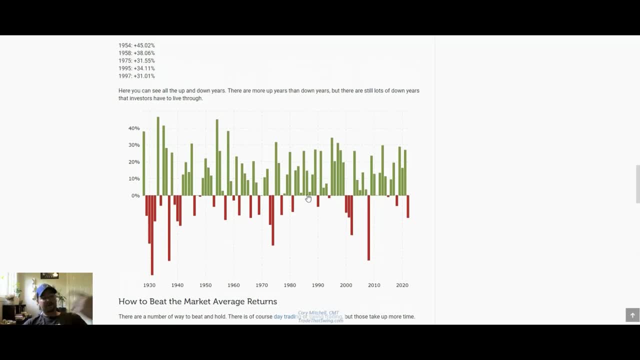 year and then ten percent on that. no, it's gonna go up and down, but over the long term it averages out to ten percent. but you could be up thirty percent when you're down to ten percent, and then 20% the next up, 15% the next. so that's how it's gonna go and so hopefully that. 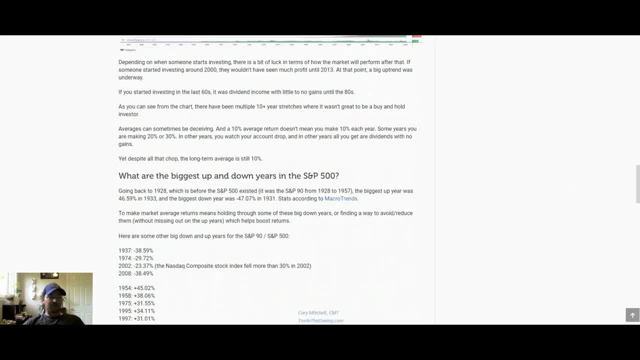 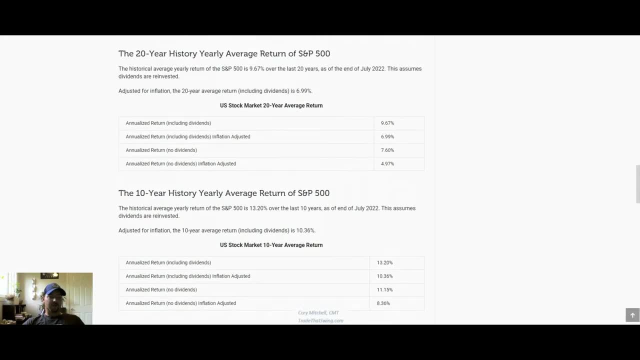 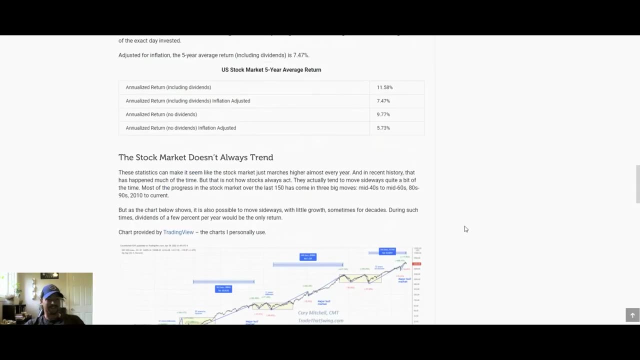 gives you an idea of what stock market history shows us about the average return of stocks, and then you can decide how you want to invest in, how you want to take advantage of that and, if you're interested in learning more about investing, how to invest throughout the year, what you should be doing to manage. 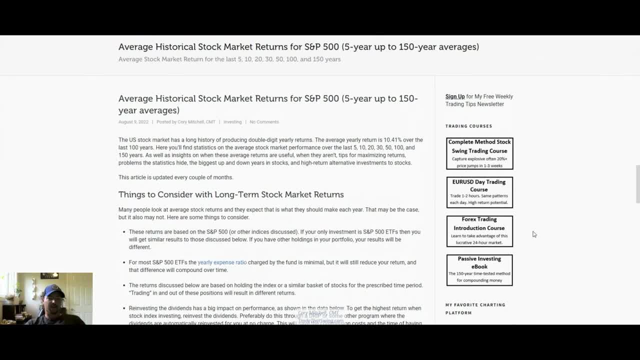 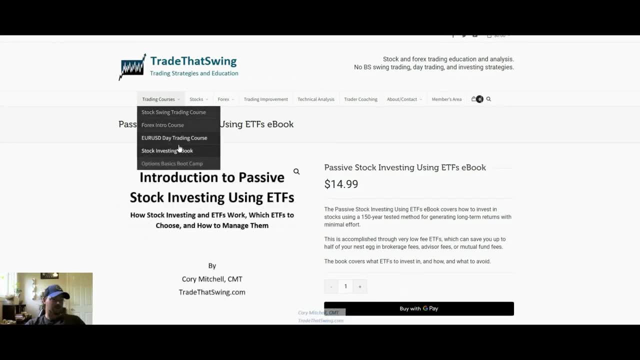 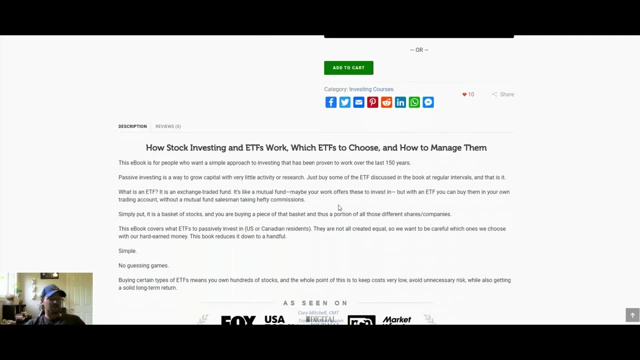 the portfolio, what funds to invest in. you can always check out the passive investing e-book. it is available on trade. that swing calm if you go to trading courses. stock investing e-book and fifteen bucks and it basically runs you through how to invest in stock ETFs and what to do with them.